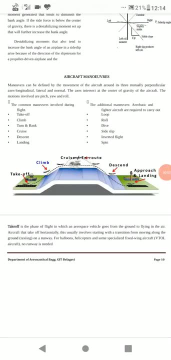 Dear students, welcome to video lecturing for the subject Introduction to Aerospace Engineering. We all know that we have covered some units in the classroom sessions, So the ongoing unit is the aircraft stability and control. in that we have started with the stability part and we have covered some of the topics. 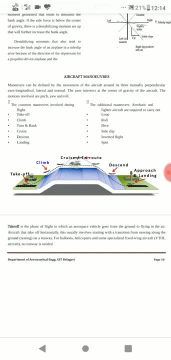 And in addition to that, in this video lecturing, we are going to cover one more topic that is related to aircraft maneuvers. Basically, the maneuver means the movement of the aircraft around its any axis. Let us say, if it is taking the help of longitudinal axis and making a movement, then it's called as roll. 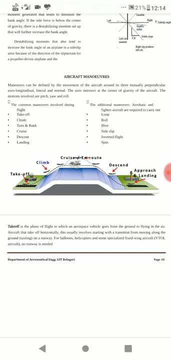 There is nothing but one kind of maneuver. Basically, these maneuvers will help the aircraft to turn, To turn around or to move forward or, you know, like to make its nose up and down like that. So in addition to that again, some more maneuvers will come, taking a low diving and side slip, those things. 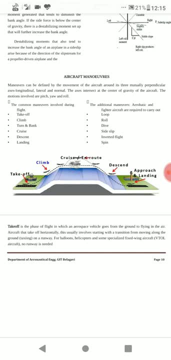 So now we will see these types of maneuvers like one by one. So aircraft maneuvers, The common maneuvers involved during flight are takeoff, climb, turn and bank cruise, descent, landing. So these are called as the basic maneuvers which are required for the aircraft. 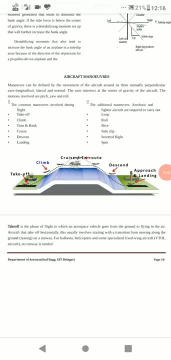 In addition to that, some fighter aircraft or fighter jets will do additional maneuvers, So they're called as loop, roll, dive, side slip, inverted flight, Spin, etc. The civilian aircraft as well as the fighter jets- all these aircraft- should undergo the basic maneuvers. 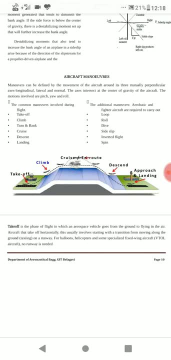 That is nothing but takeoff, climb, turn and bank cruise, descent, landing And basically these common maneuvers are around the axis, different axis. For an example, takeoff and landing is nothing but the pitching moment we can say. 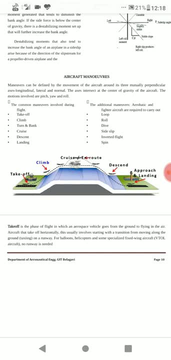 That means while taking off, it has to make the aircraft nose upward direction And while landing, it has to make the aircraft nose in downward direction. That means the movement is happening with respect to the lateral directions. So, similarly, if it is turning and banking, that means it has to roll. 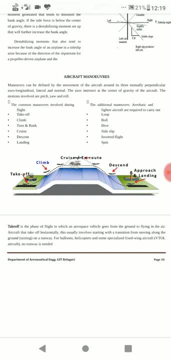 And that will happen with respect to the longitudinal axis. And while cruising time, what will happen? It has to change the direction. Then the movement or the maneuver will happen with respect to the directional axis. Now we will understand why these maneuvers are required. 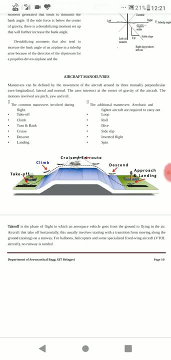 The pilot must have enough knowledge about maneuvers, Otherwise he cannot become a good pilot. So why it is required? basically, For an example, you take an incident. Let us say the aircraft is landing in the Bangalore airport, But the ground people who are there, the technicians or the ground communication people, will say to the pilot: 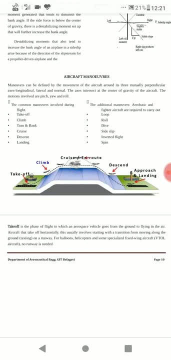 like here. the runway is busy So you need to keep on rounding in the air. That means the pilot has to take or do some maneuvers in the air itself. Then he can land. So these kind of critical situations will come. So there is a reason. 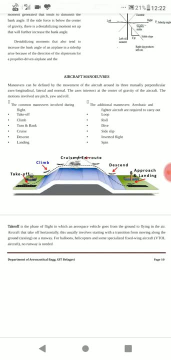 The pilot must know, You know like, the maneuvering techniques. So, apart from him, the fighter jet, especially the aircraft which is used for military purpose There, the pilot must know the additional maneuvers also. So in order to escape from the enemy, or to put the bomb or something else, 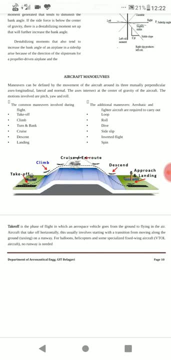 In this video we will cover this much, And in upcoming video we will talk separately with respect to the additional maneuvers. Thank you,